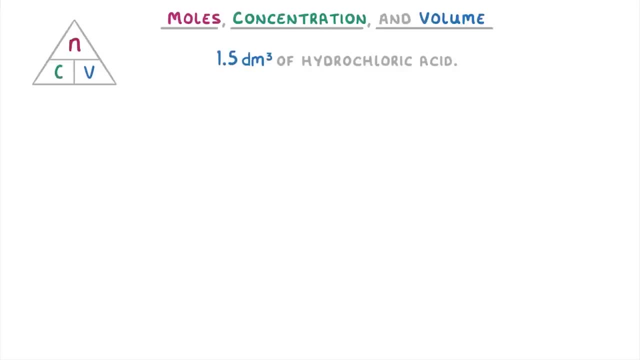 five decimetres cubed of hydrochloric acid and we're told that it contains zero point six moles of hydrochloric acid. What must the concentration be? Well, if we look at our equation, concentration is moles divided by volume, And as they're both already in the right units, 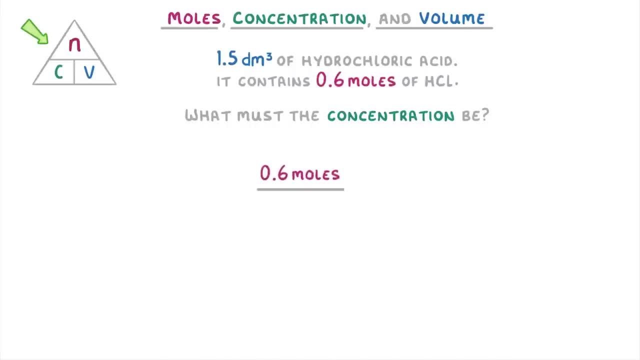 we just do zero point six divided by one point five, which gives us a concentration of zero point six moles per decimetre cubed. concentration of 0.4 moles per decimetre cubed. Now, a more complicated scenario is when we're given an equation like this one. 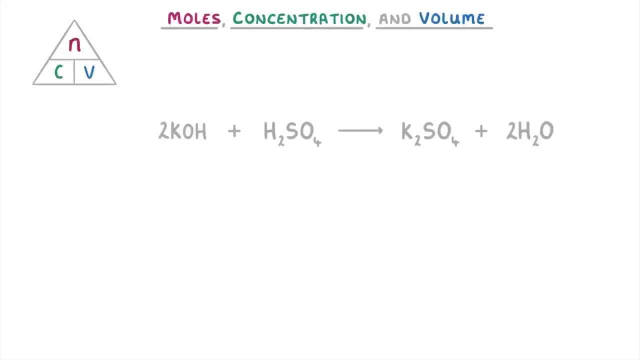 here and we're asked to find an unknown concentration or volume. For example, if we knew that 30 centimetres cubed of 0.5 mole per decimetre cubed potassium hydroxide reacted completely with 25 centimetres cubed of sulfuric acid, we 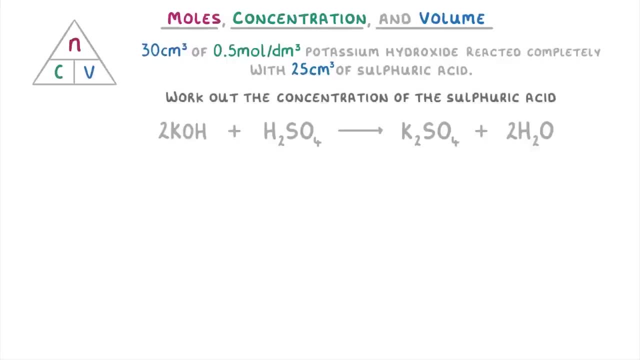 should be able to work out the concentration of the sulfuric acid. Before we do anything else, though, it's worth writing out clearly what we already know from the question. For the potassium hydroxide, its volume is 30 centimetres cubed and its concentration is 0.5 moles per decimetre cubed. 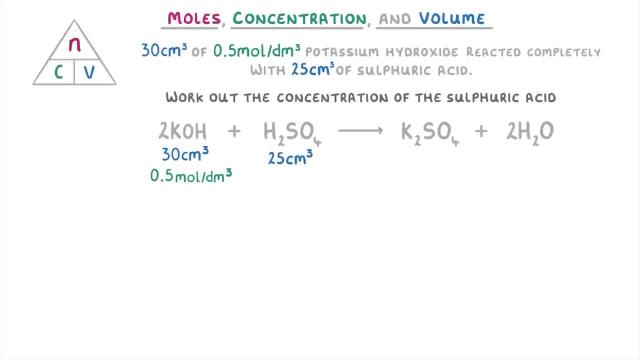 And for the sulfuric acid, we know its volume is 25 centimetres cubed. Then, because this is a chemistry calculation, we know that we're going to need all of our volumes in decimetres cubed and not centimetres cubed. So we 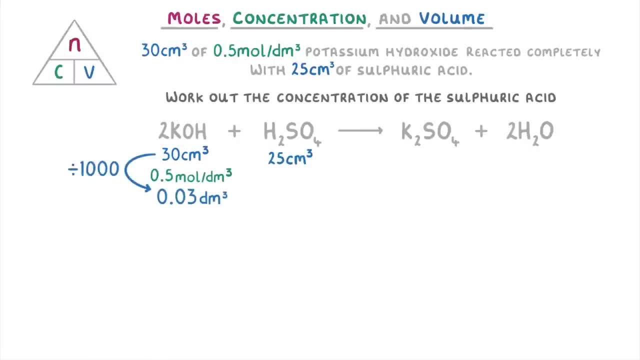 divide 30 by 1000 to get 0.03 decimetres cubed, and 25 by 1000 to get 0.025 decimetres cubed. Now the basic question is: how do we know the concentration of 0.5 moles per decimetre cubed? 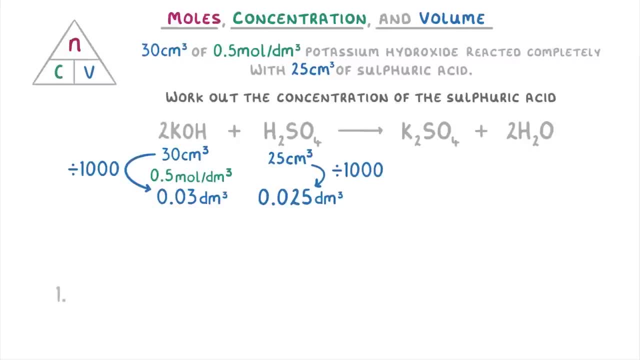 The basic idea with all of these types of questions is first to work out how many moles of the known substance we have, Then, second, use the molar ratio to work out how many moles of the unknown substance we have, And finally, use that number of moles to work out the concentration. 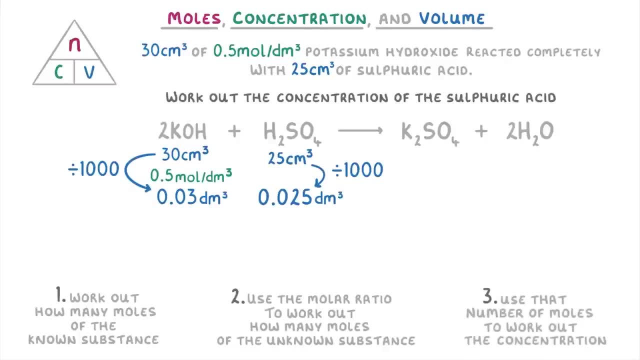 of the unknown substance. So our first step is to calculate how many moles of potassium hydroxide we have, which we can do by multiplying its concentration by its volume. So we do 0.5 times 0.03, meaning we have 0.015 moles of potassium hydroxide. Then for our second, 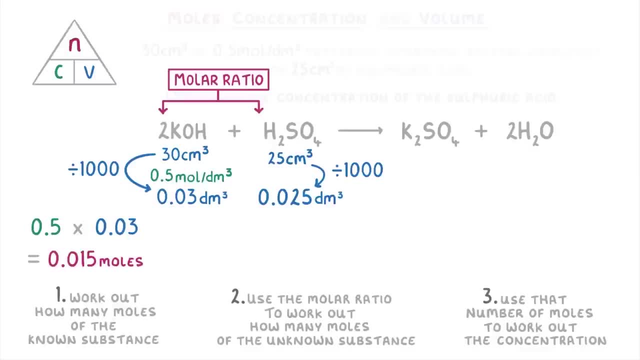 step, we need to find the molar ratio between potassium hydroxide and sulfuric acid, which we can do by looking at the numbers in front of each of them And remember that if there isn't a number before the substance, like for the sulfuric 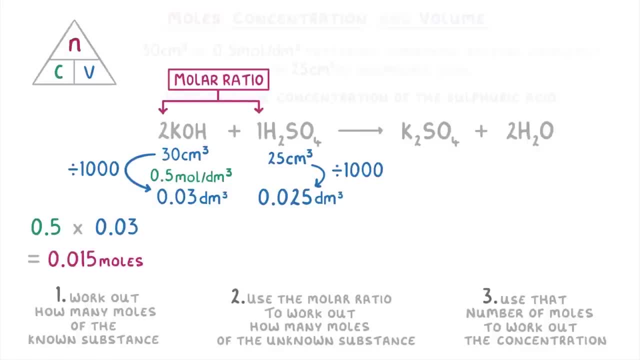 acid, then we just read it as a 1.. So the molar ratio here is 2 to 1, which just means that for every 2 moles of potassium hydroxide we'll have 1 mole of sulfuric acid. So because 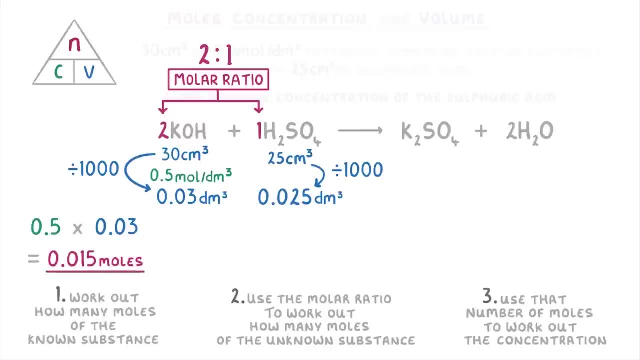 we just worked out that we have 0.015 moles of potassium hydroxide. then we just need to divide that by 2 to find out how many moles of sulfuric acid it reacted with, giving us 0.0075 moles of sulfuric acid, And finally we can move onto our third step, which is: 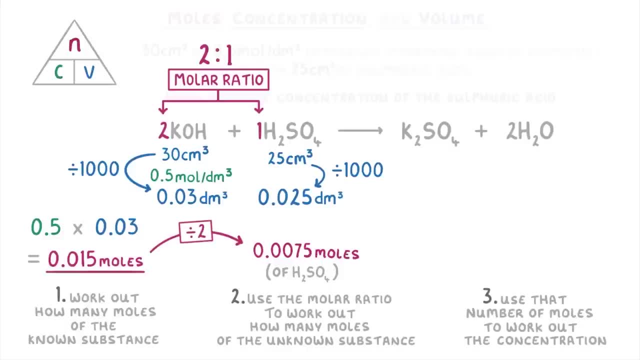 where we actually calculate the concentration, using the number of moles that we just found and the volume that we were given in the question, which, remember, we converted here to 0.025, decimetres cubed. So we take our 0.0075 moles of sulfuric acid and divide it by the volume. 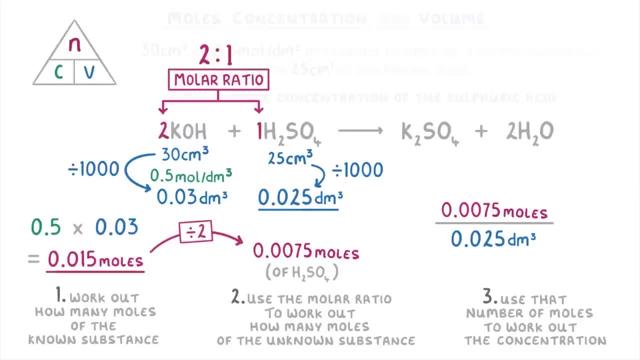 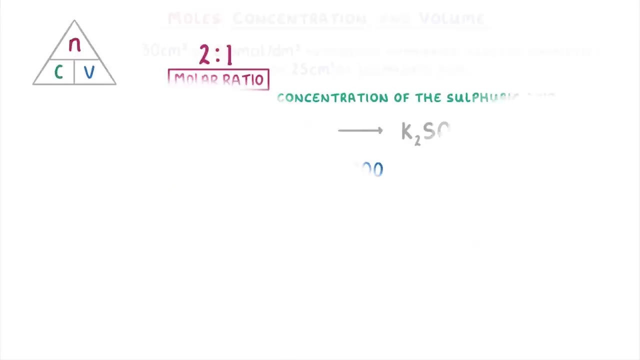 of 0.025, which tells us that the concentration of sulfuric acid is 0.3 moles per decimetre cubed, And that is our final answer to the question. Anyways, that's everything for this video, so hope that all made sense and we'll see. you again soon.